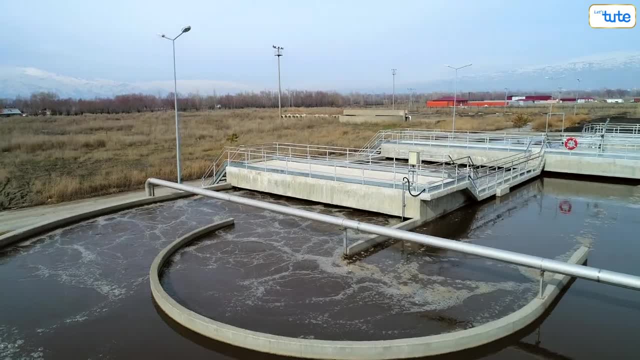 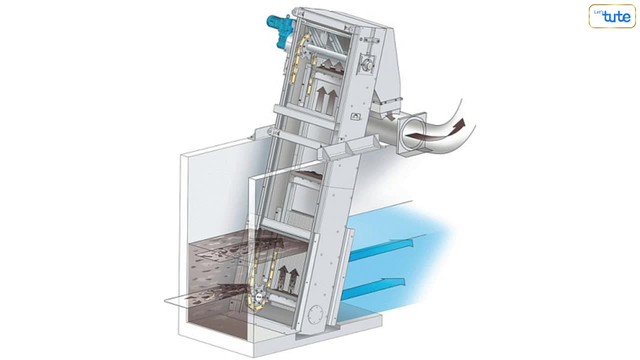 next, Make sure you watch the video till the end. The first step in the wastewater treatment process is screening. The physical process of wastewater treatment begins with the treatment of large items that have found their way into the sewer system and, if not removed, can damage pumps. 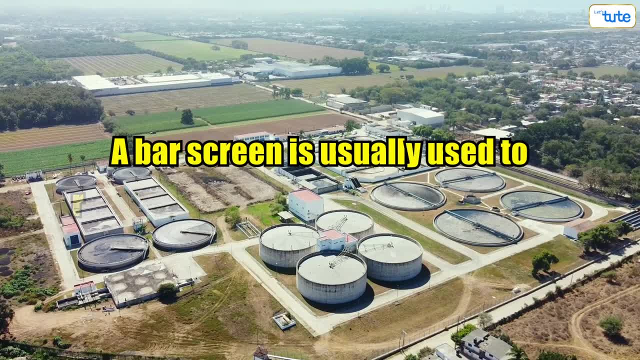 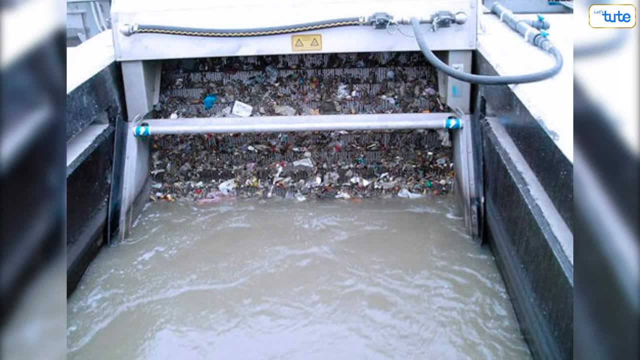 and impede water flow. A bar screen is usually used to remove large items from the influent and is ultimately taken into landfills. This is like a filter that catches large items like sticks, rocks and trash, But smaller and fine grids can easily make their way through the bars and can. 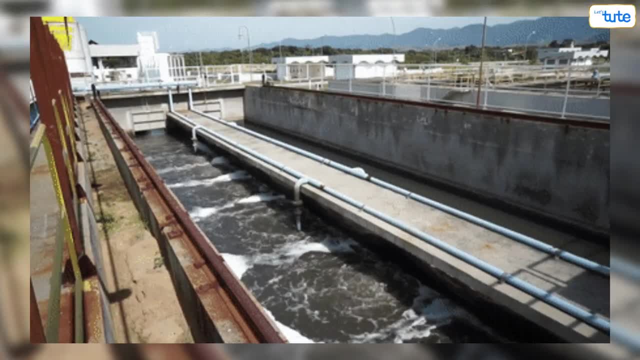 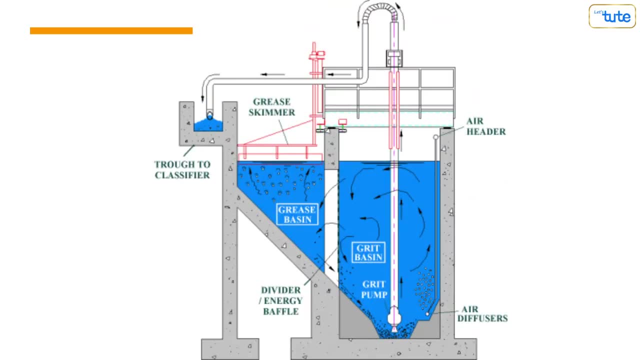 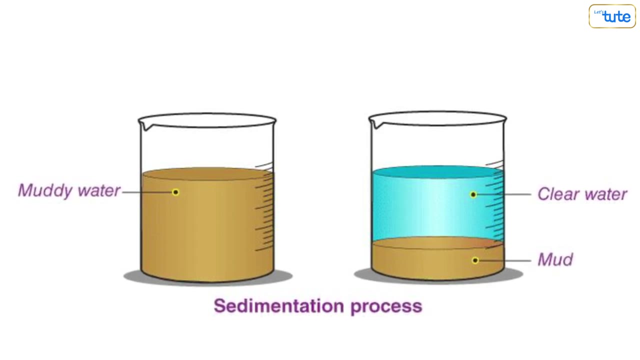 damage the pumps and the other equipment. Too small to be screened out. this grid needs to be removed from the grid chamber. So the second step of wastewater treatment is grid removal. The third step is called sedimentation. In simple terms, it is a process of settling after grid removal. The 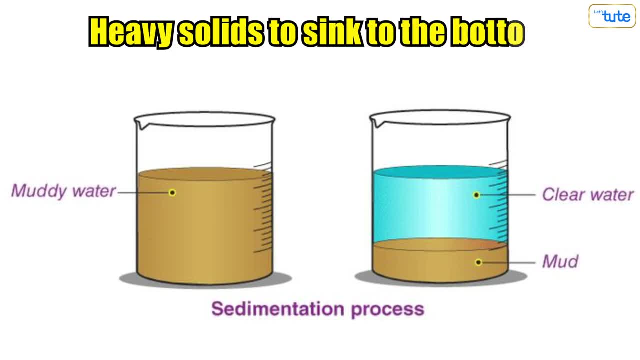 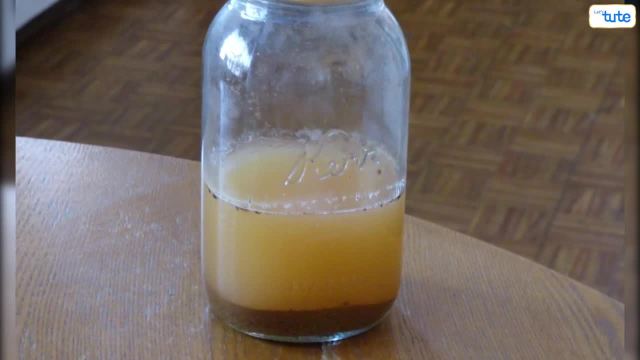 influent enters the large tanks that allow the heavy solid to sink into the bottom and cleaner influent to flow. The solids that fall to the bottom of the tanks are known as sludge and are pumped out regularly to ensure it does not impact the process of separation. The sludge is then 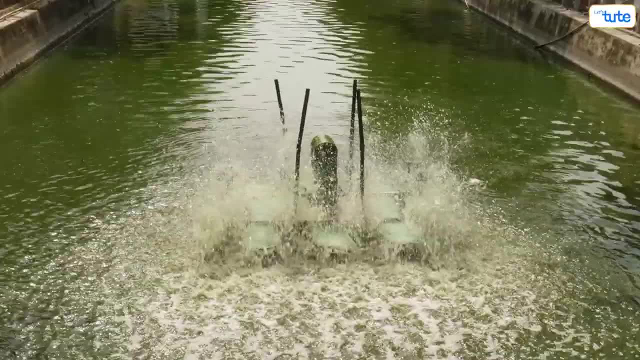 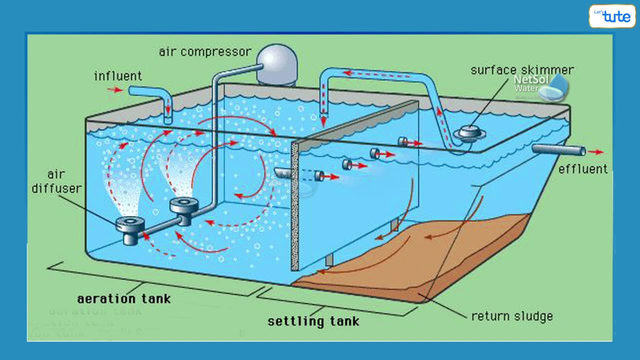 discarded after all, the water is removed and commonly used as fertilizer. The fourth step is called aeration. After the separation of all the solids, the wastewater is now put into the aeration tanks. As the name suggests, air is pumped into the tank. This 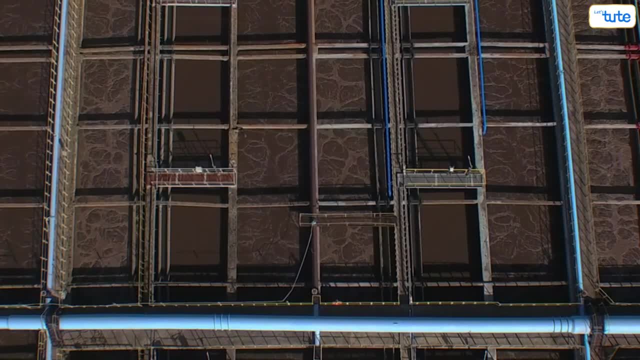 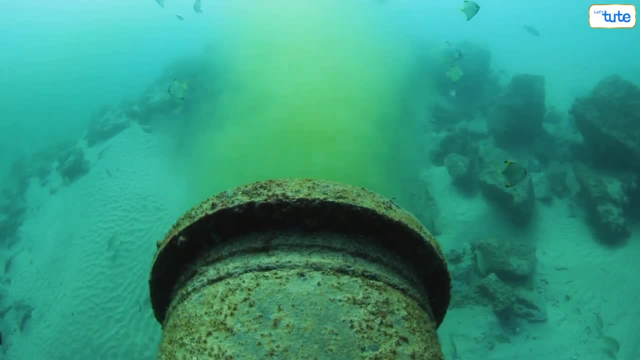 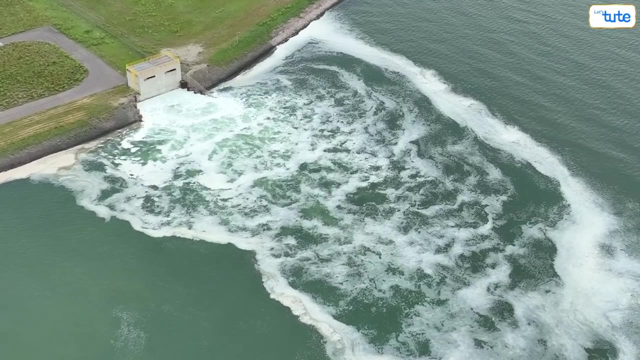 provides oxygen for bacteria to continue to propagate and grow and further break down to the organic matter present in the wastewater. The organic matter content of wastewater discharged into nearby streams determines how much oxygen will be available for the fish to breathe, Meaning, if the wastewater has too much organic content, all the oxygen would be. 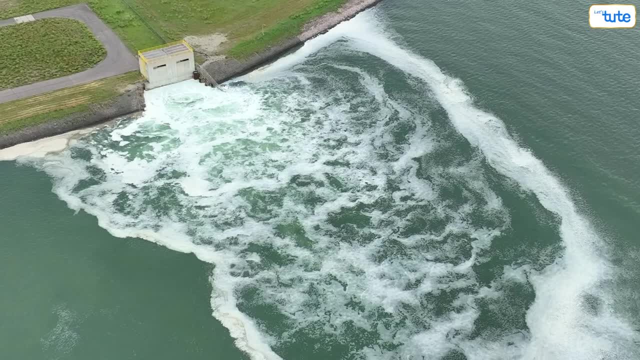 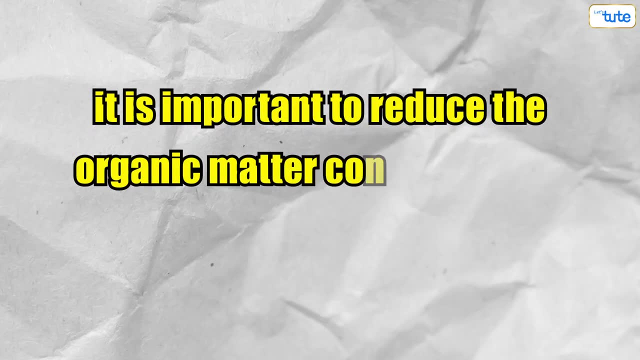 utilized for its breakdown and the oxygen supply for the aquatic organism would be limited, thus increasing the biological oxygen demand. Hence it is important to reduce the organic matter content before discharging the wastewater Now, to further accelerate the breakdown of the organic matter. 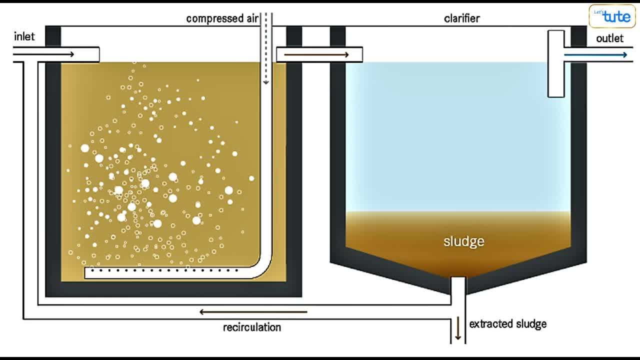 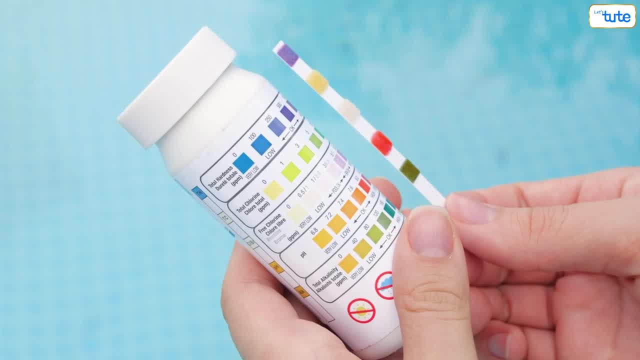 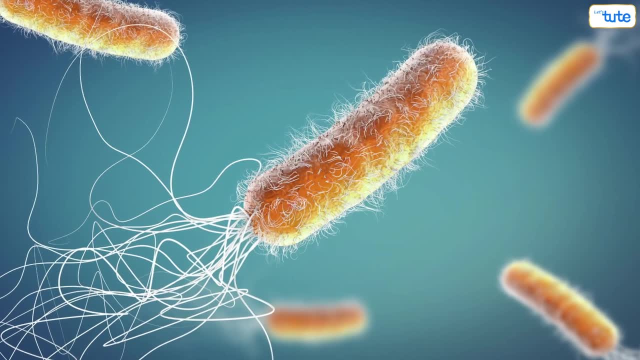 the water from the aeration tank now moves to another tank which is loaded with small solids called activated sludge, which consists of concentrations of bacteria. The final step is disinfection. This is where chemicals like chlorine or ultraviolet light are used to kill any remaining harmful bacteria and viruses.